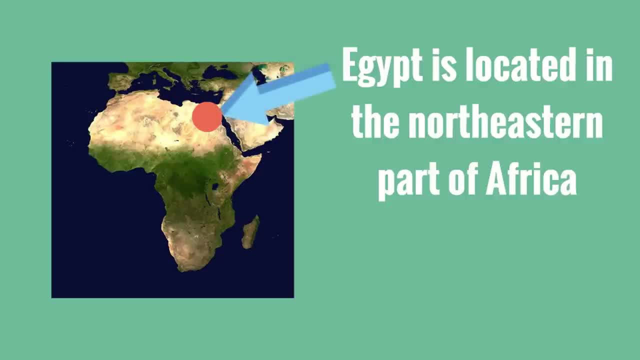 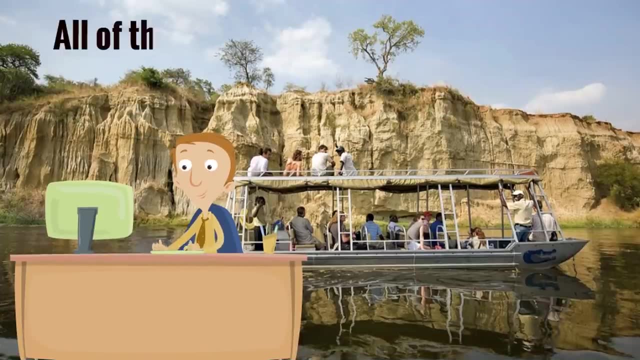 it's in the northern part, It's in the eastern corner. That's where Egypt is. You can see it right here. Interesting fact: you might not know, but all of the early civilizations were near rivers. Look at this river. All of the early civilizations were near rivers. Now why do you think they? 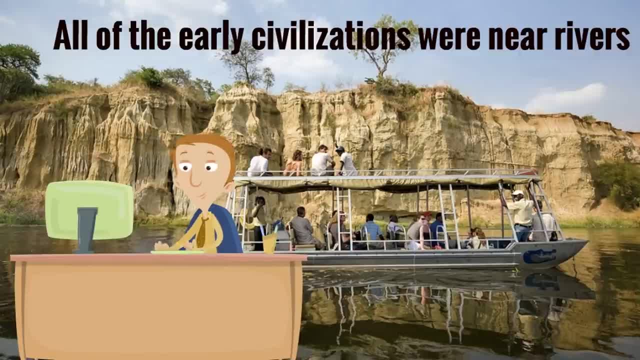 were near rivers. Why would you build a civilization around a river? Why do you think, Yeah, because of the water You need. the water for the crops and for drinking Water is life, And in some of these climates, you really needed to be near that water in order to survive. And so all of the early civilizations. 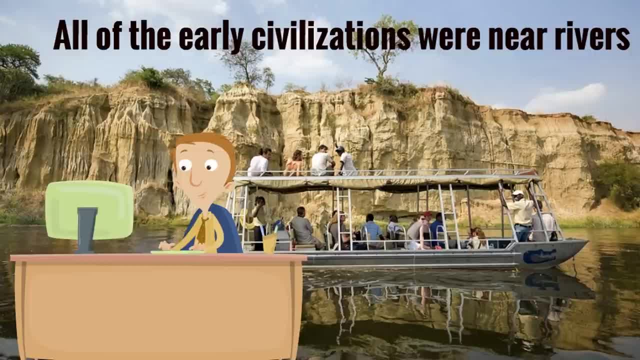 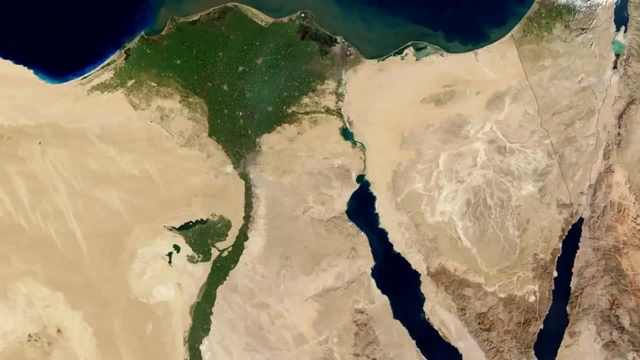 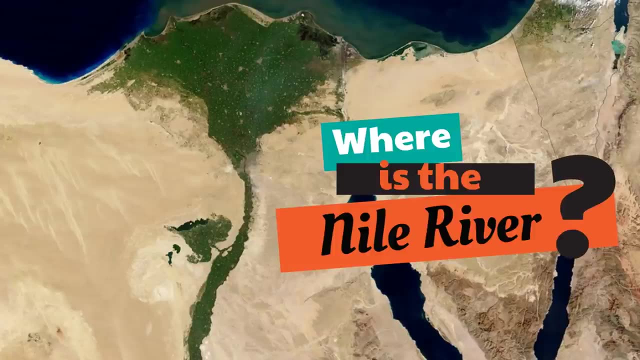 were near rivers. Ancient Egypt was no different and was near the Nile River. Now look at this picture of where ancient Egypt was. Where do you think the Nile River is? It's kind of interesting because when you have water it helps plants grow. 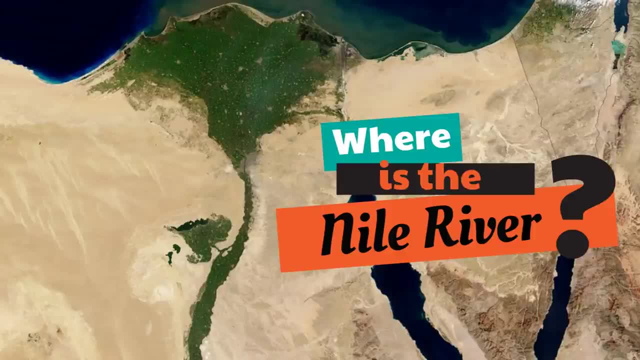 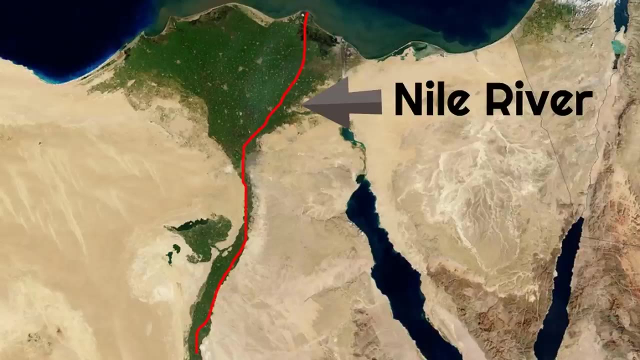 What do you notice? Do you see a line, especially on the bottom, near the bottom? from the top, You see lots of green on the top and then you see a line of green. Why do you think that is? Yeah, the Nile River is watering all those plants and that trail is the Nile River. 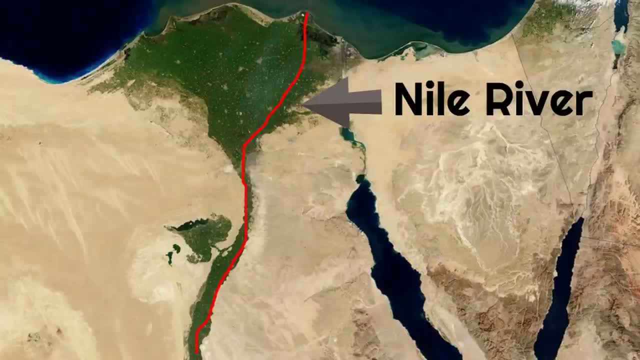 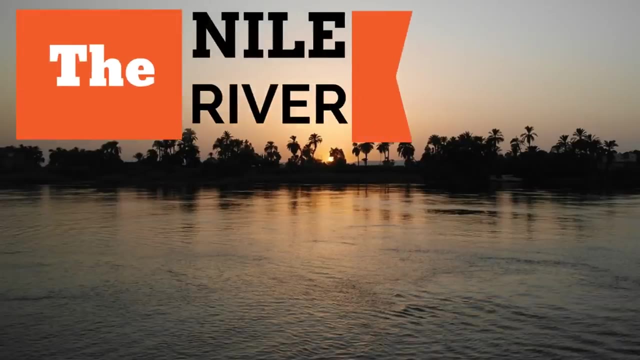 The Nile River is actually in that upper part as well, with all that green, But it's interesting the lower you go into Egypt. what's neat is you can actually see the trail of the river just by looking at the plants. There it is, There's the Nile, and it still helps people today. This water made it possible for 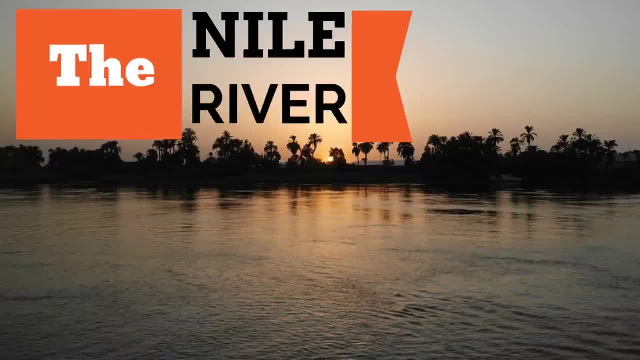 ancient Egypt to even exist as a civilization. Yeah, the Nile River. Can you say that with us? Say Nile River, That wasn't loud enough. Come on Say Nile River. Yeah, the Nile River, The Nile, The Nile. When you think Nile River, think, oh my goodness, that's what allowed ancient 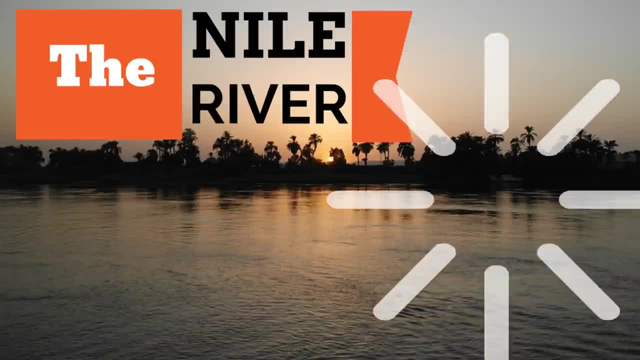 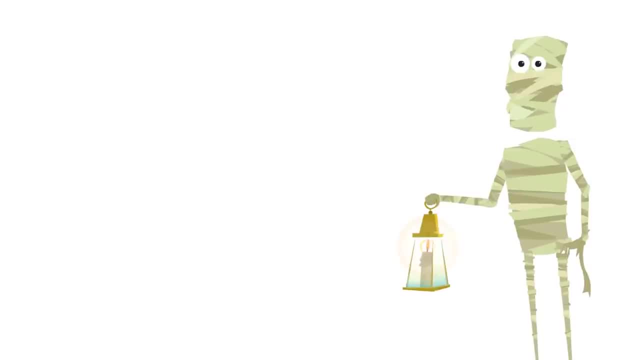 Egypt to be a great civilization. The Nile River- Wow, The Nile, Do you mind? I mean, I already told you we're going to talk about you. okay, It's about ancient Egypt. We got to talk about mummies. All right, We're still talking about the Nile. You could have. 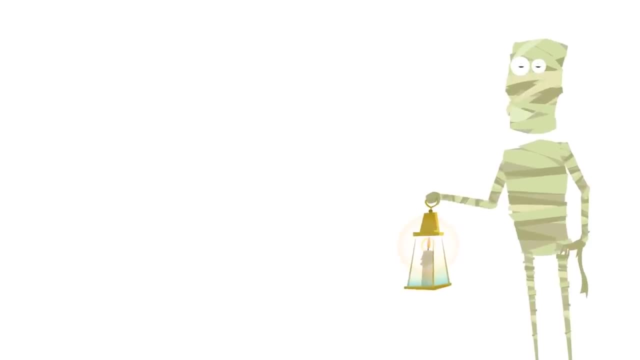 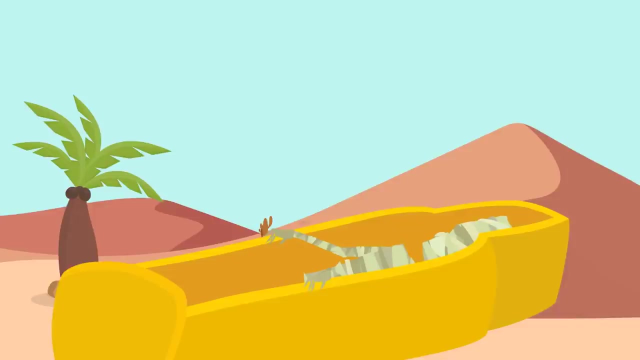 waited your turn. All right, Just get back. in your case, Do whatever you like to do. Okay, Now you're just being creepy. okay, This is for kids. all right, You need to behave, or you're just not going to be on this one. okay, You're just not. And if you're not on this one, 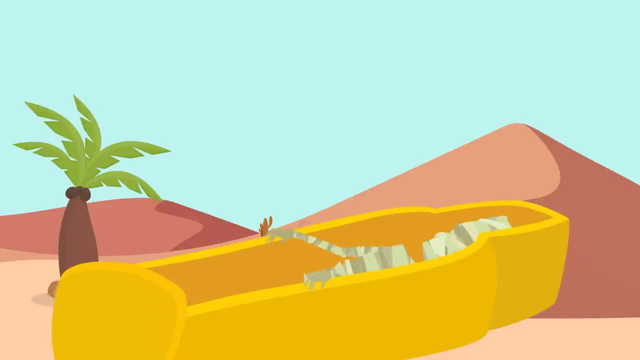 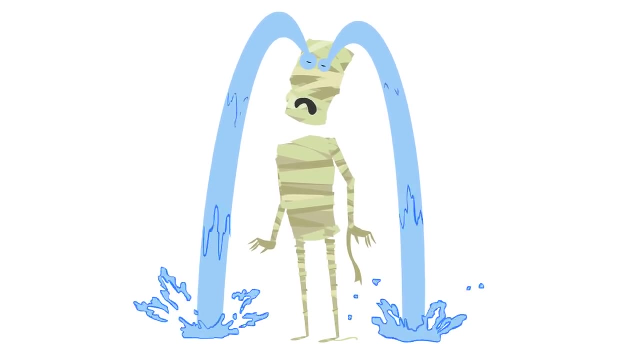 listen, we don't have mummies on our other videos. This is your one shot. You need to behave. Oh wow. Oh man, I didn't know you were going to be so sensitive. I didn't know that you were. I didn't know you had feelings. You're a mummy. I just 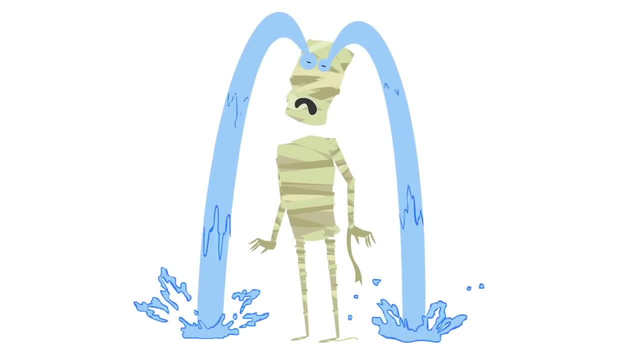 I didn't know. Listen, all right, You can be in it. You can be in it, all right. Just no more of this crying stuff. okay, You're in it. okay, You're going to be in it, all right. 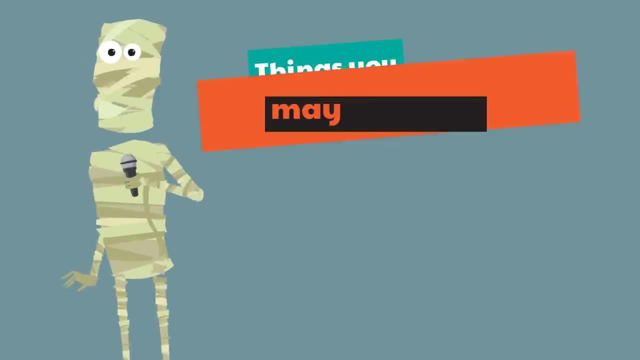 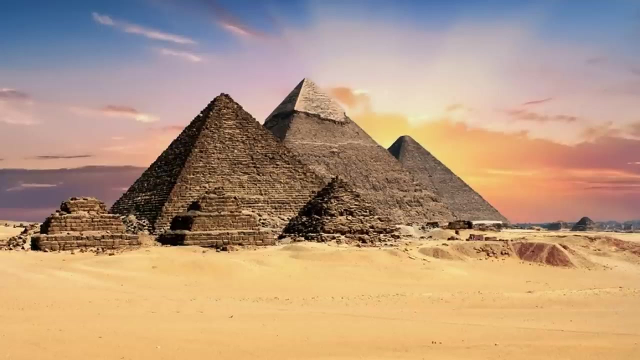 Let's just move forward. all right, Okay, good Happy. All right, Awesome. Now here's some things you may already know about ancient Egypt. This is part of what made ancient egypt so famous. what are these? do you know what these are called? 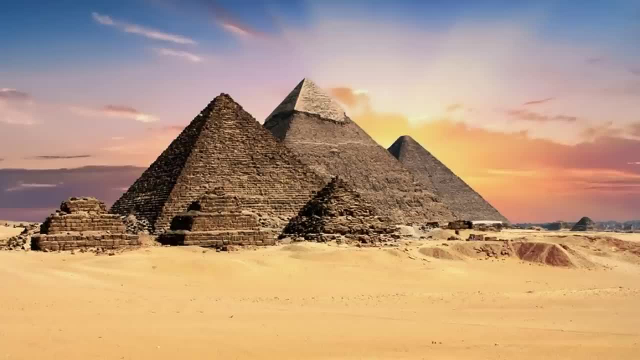 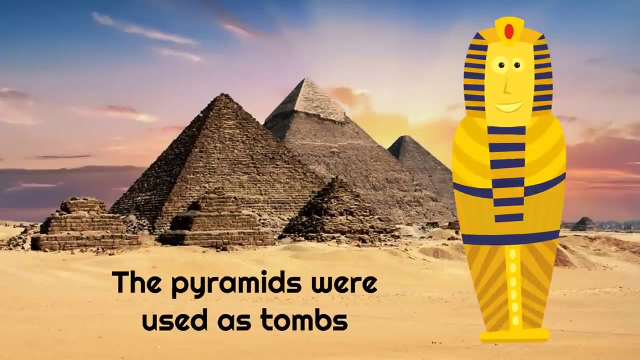 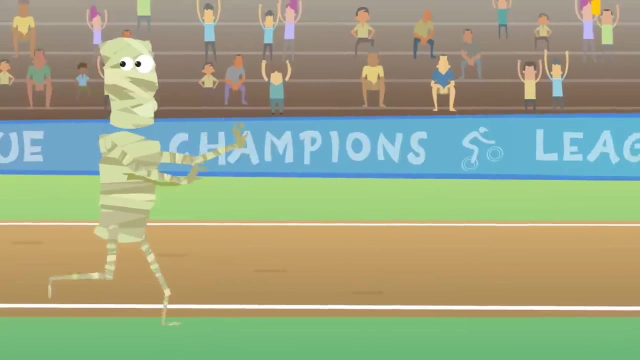 yeah, they're called pyramids. it's pretty cool that, even though they were built so long ago, they're still standing today. the pyramids were used as tombs. when someone important in the society died, they might be placed in a pyramid. they would preserve people's bodies through a process called mummification.